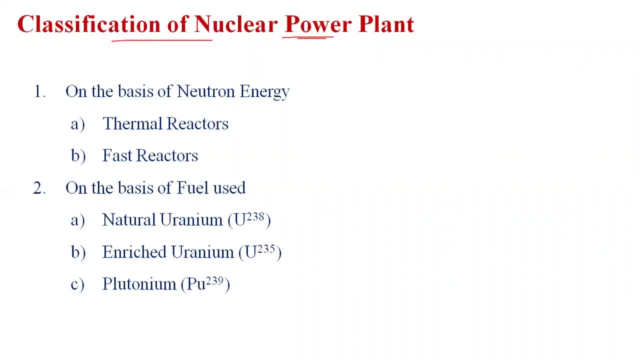 power plant. various types of nuclear reactors used, classified into five types In that the first one, the basis of neutron energy, based on neutron energy. Here there are two types of the reactors used in the neutron energy. One is for the thermal reactor, another one 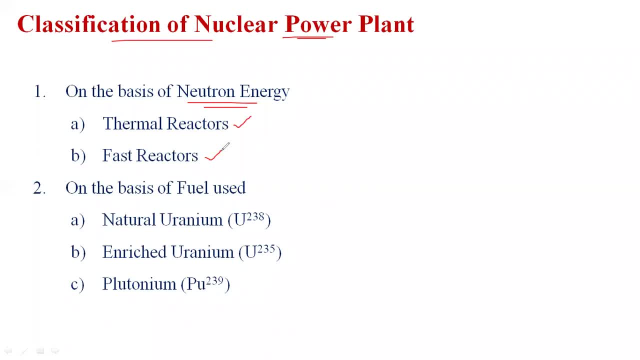 is for the fast reactor, Thermal reactor, another one is for the fast reactor. In the thermal reactor the moderator is used, but in the faster reactor the moderator is not used. Actually, in the nuclear power plant, once the fission process is taken place, Then 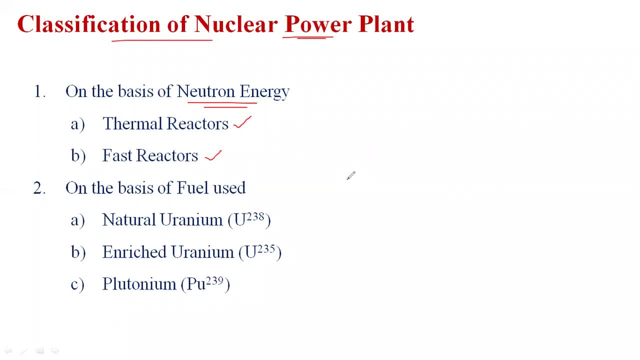 if the fuel is used uranium, thorium or plutonium, once the fission process is appeared it reaches for radioactive substances. Generally, in that we are using for the moderator, it observes some amount of the radioactive substances in the reactor. That means once some Wet. 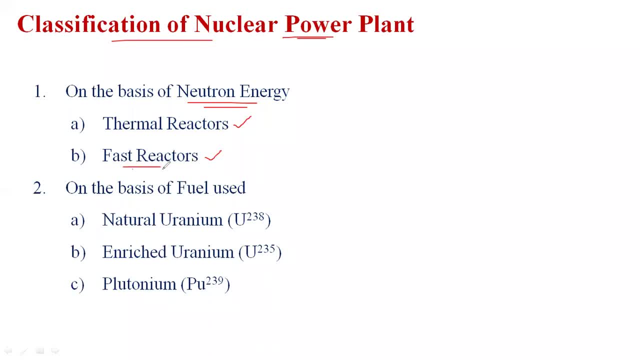 substances. If you are not used for the moderator directly it releases for the first neutron In that the radioactive substances is entering to the atmospheric particle. But maximum in the nuclear power plant they are preferred. for the thermal reactors They are preferred. 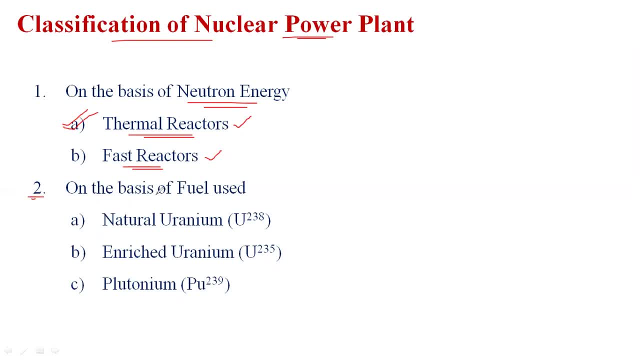 for thermal reactors, The second one. it is preferred on the basis of fuel used In the nuclear power plant. the fuel we are using is uranium thorium and then plutonium, Uranium thorium and then plutonium, But maximum they are preferred for the uranium Another. 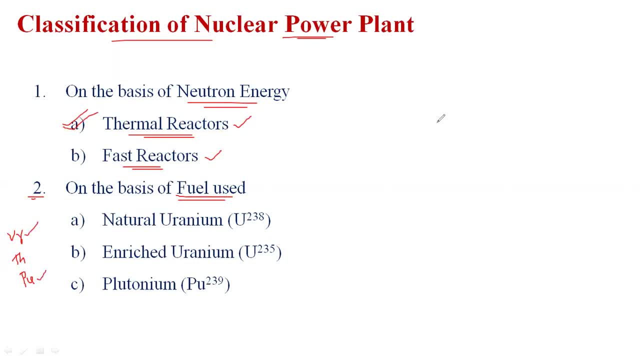 one is for the plutonium. Again, in uranium, it is classified for two types of fuel. One is for the natural uranium, Another one is for the enriched uranium. Natural uranium, the number is represented for 238, and the enriched uranium, that is 235, and the plutonium. 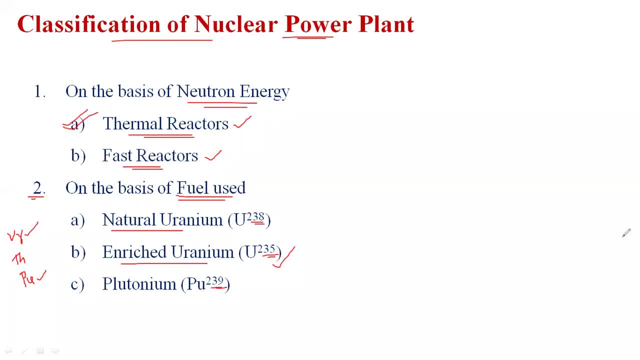 is 239.. But maximum in the nuclear power plant. they are preferred for the plutonium In the enriched uranium, that is uranium 235.. Actually, in the enriched uranium the efficiency we are getting is maximum And another one the fuel utilization, that is, the consumption. 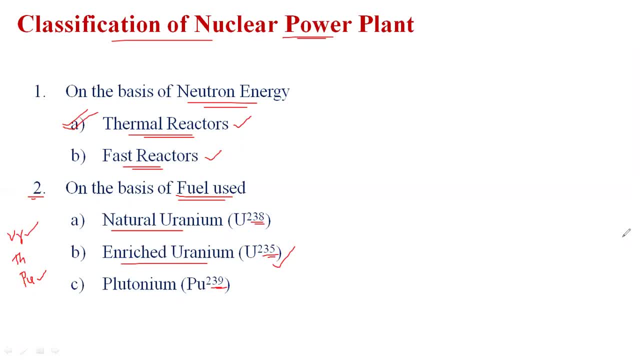 is also somewhat less Because here the wastage particle is very, very less. Once we are using fuel we are getting more than 85 percentage of the efficiency, comparing to the natural uranium and the plutonium Maximum- all the nuclear power plant they are preferred for. 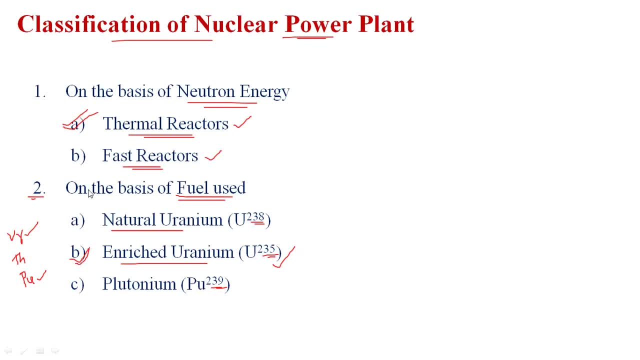 the enriched uranium: Enriched uranium And the next classification based upon the moderator used. Moderator used Actually here the moderator. the particulars they are used is graphite reactor, heavy water reactor, ordinary reactor, beryllium reactor and last one is: 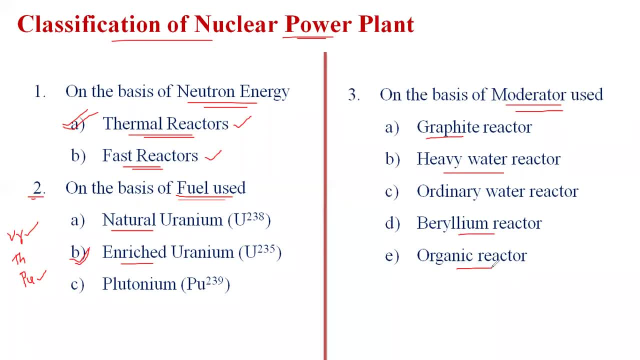 organic reactor In the nuclear power plant. they are preferred only for the graphite reactor And that is the graphite material. It is not released for the open atmospheric. that is this radiation particle, that is radioactive substances, If in the reactor core it is. 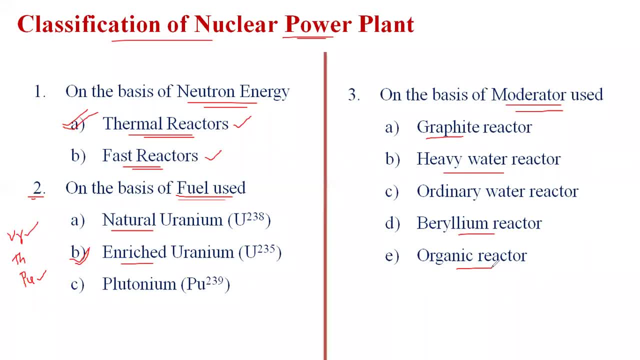 any alpha particle or beta or gamma radiation released means this graphite particle is observed and it is not reflected into the open atmosphere. It is not fed back into the open environment Generally the moderator, the material. they are used for the graphite reactor, So the 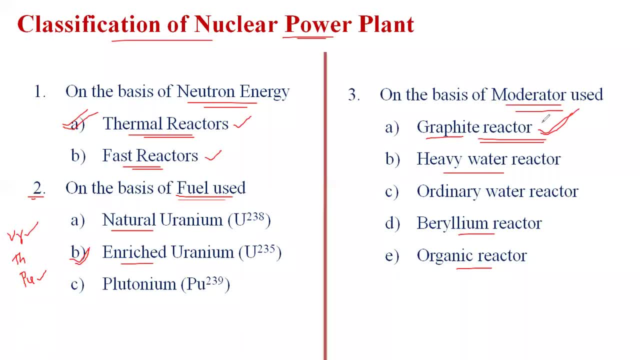 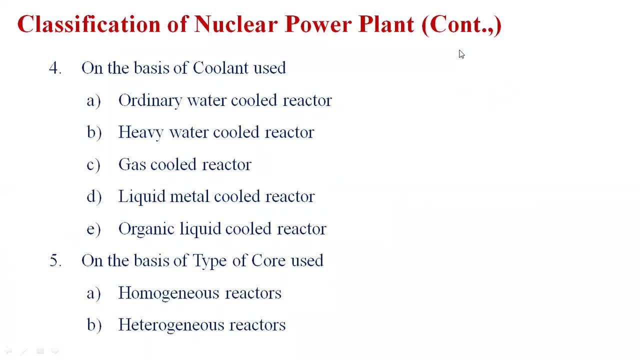 material is graphite material in the nuclear power plant. And the next classification is on the basis of coolant. On the basis of coolant- This is used in the moderator- There are ordinary water cooled reactor, heavy water cooled reactor, gas cooled reactor, liquid metal cooled. Another one is for the organic liquid cooled reactor. 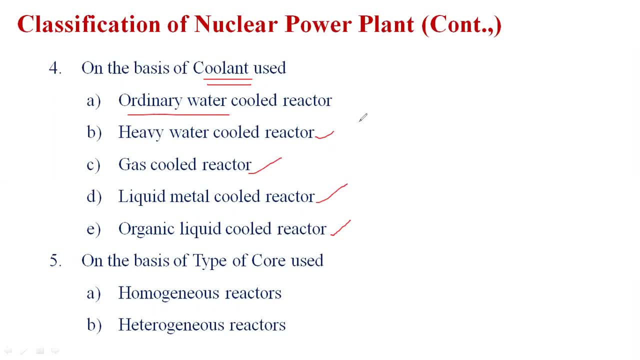 Actually, in the nuclear power plant the initial or capital cost is very, very high. So the material is graphite material and in the nuclear power plant the material is high and the fuel cost is maximum. fuel cost is maximum for coolant purpose if you go for the. 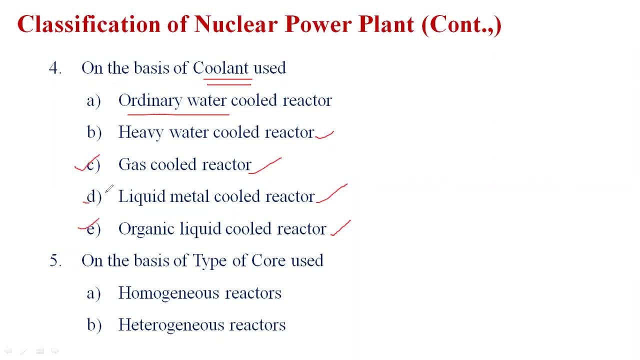 gas cooled reactor or organic liquid or liquid metallic cool. again the cost is increased. at present the per unit cost we are generating in the nuclear power plant it is more or less around 20 rupees. same we are compared in the renewable energy sources, that is, solar power plant. the per 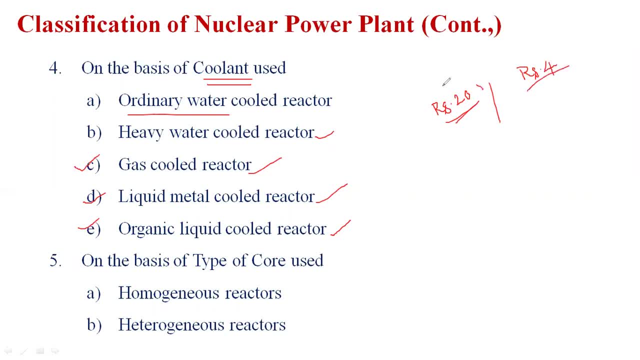 unit cost is comes under only 4 rupees if the same power we are generating in the thermal power plant. the per unit cost is comes under for either 3 to 5 rupees- 3 to 5 rupees, but here the per unit cost. 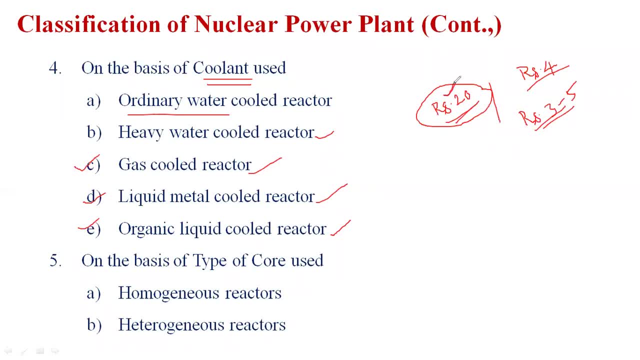 is high. actually, the main objective of the power system is we need to satisfy for the consumer two parameter: one is for the quality, another one is for the quantity. quality means without interruption and without load fluctuation. quantity means a Here the cooling purpose, if used for the gas cooled reactor, means again the burden is presented. 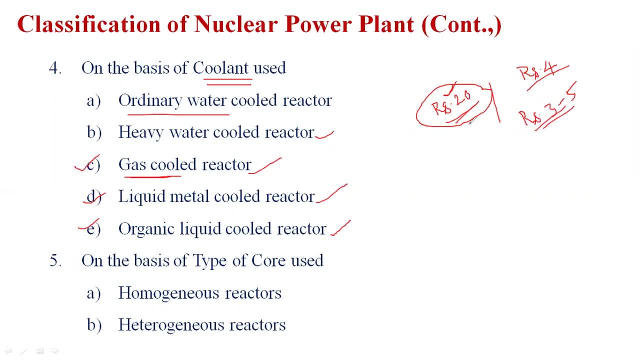 for the consumer. Again the cost is increased. Again the per unit cost is increased 21 rupees or 22 rupees. The consumers are not satisfied. For that purpose, the coolant in the nuclear power plant, they are preferred for the ordinary. 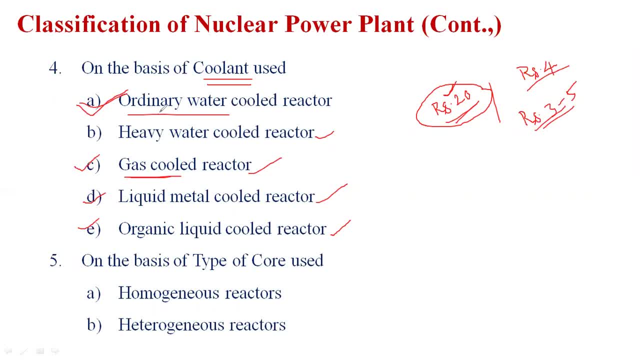 water cooled reactor- Ordinary water cooled reactor- And the last one on the basis of type of core used. on the basis of type of core used Here. there are two types of core used here. One is something for the homogeneous reactor, another one is for the heterogeneous reactor. 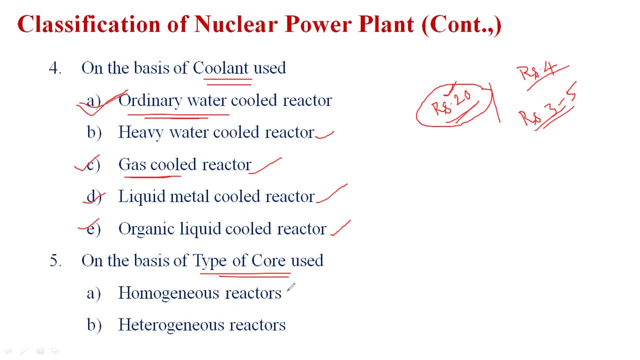 Here the type of core is classified for two types. One is for the homogeneous reactor, another one is for the heterogeneous reactor, But maximum in the nuclear power plant they are preferred for the homogeneous reaction. homogeneous reactors. These are the various classification of the nuclear reactors in the nuclear power plant. 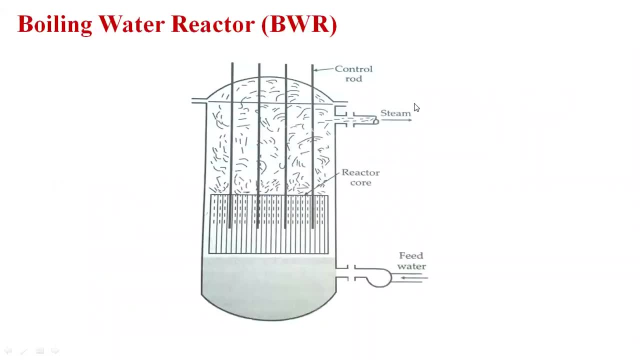 Next topic is the nuclear reactor. it is classified for three types. One is for the boiling water reactor: it is represent for BWR. The second one, pressurized water reactor, that is PWR. And next one is nothing but the fast breeder reactor, that is represent for FBR. 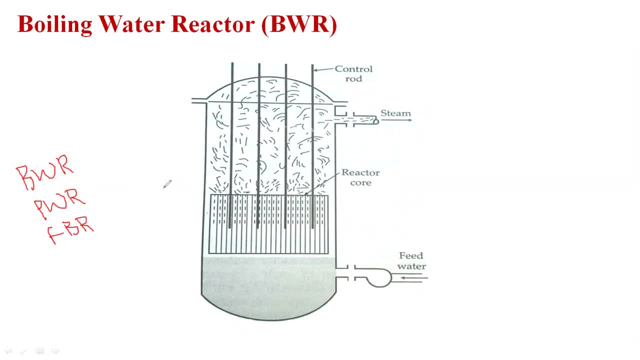 Generally in the nuclear power plant the nuclear reactors are classified into usage. they are classified into two types. One is for boiling water reactor. that is represent for BWR. Pressurized water reactor is represent for PWR. Another one, fast breeder reactor, is represent for FBR. 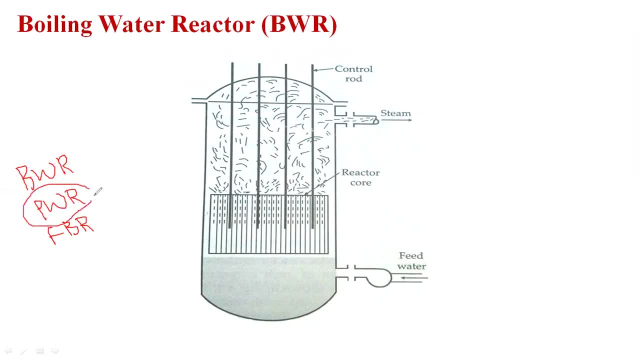 But in the nuclear power plant they are preferred for the pressurized water reactor PWR. Why they are preferred pressurized water reactor. this we can go through it In that the first one is the boiling water reactor. This is one of the simplest type of water reactor. 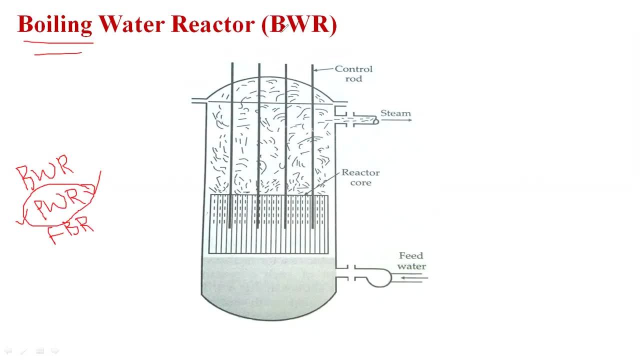 Here the PL used is enriched reaction. Here the boiling water reactor. the PL used is enriched uranium. That is the enriched uranium it is represent for uranium 235.. Here it is used for both. that is, the moderator and the coolant purpose. 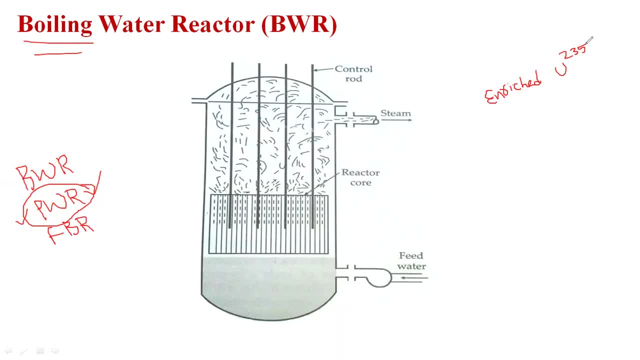 This boiling water reactor water is used both moderator and coolant. In this case the steam is generated in the reactor itself. Here they are not used for the moderator Only, they are used only for the reactor. In this reactor itself the steam is generated. 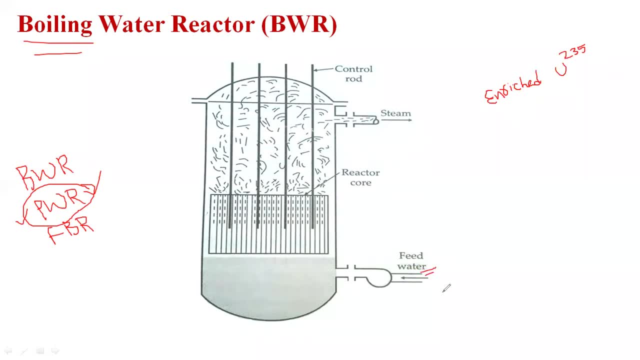 That is the fed water. the fed water, that is the water- is carried from the fed water pump. The water is carried from the fed water pump entering to the reactor tank at the bottom. That is the bottom, the water it will be entering. 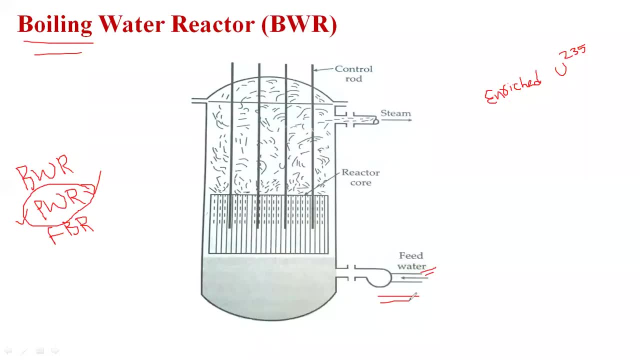 And the heat generated due to the water is generated. The heat generated due to the fission process. The heat generated due to the fission process based upon the control rod. Whenever the control rod is pushed towards the PL, some amount of the fission is observed. 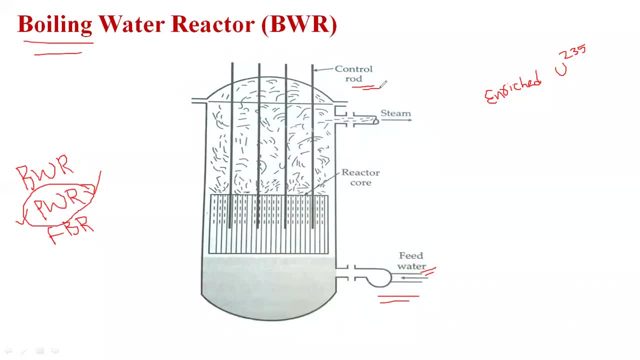 That is, only few neutrons are released. Whenever the control rod is pulled out, that is pulled upward, more number of fission is released. The power generation is maximum Based upon the demand. it can control the power generation based upon the control rod. 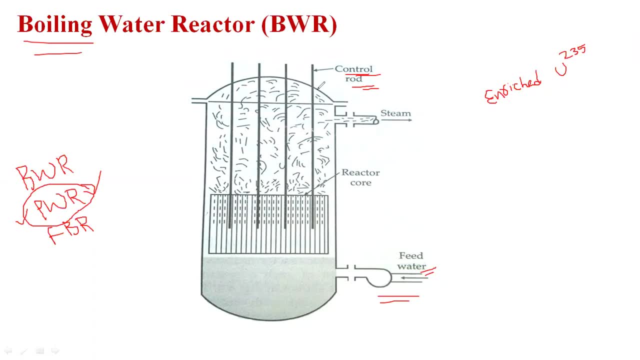 Here the steam is generated during the fission process And converted into steam. the steam leaves the reactor at the top- The bottom we are supplying the fed water And the top we have taken for the steam. This steam drives the steam turbine, which converts the steam energy into mechanical energy. 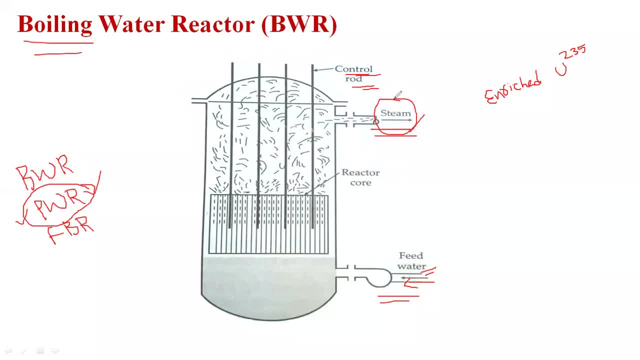 Further that mechanical energy converts into electric energy with the help of alternator. With the help of alternator, Again, the wastage steam collected in the condenser again circulated to the reactor In the form of fed water. And here the water and then the steam, the both it will be merged to each other. 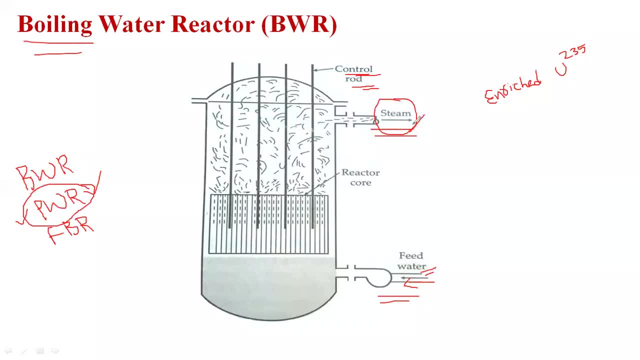 Here. they are not used for the moderator Here. one main drawback is there: Directly it releases the steam in the reactor itself That drives the steam turbine. If any radioactive substances are entered, it enter into the environment. It polluted to the environment. 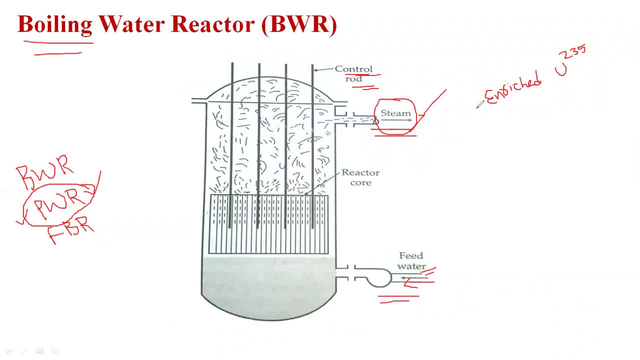 It polluted to the environment. And one more drawback: it cannot meet sudden increasing in load. It cannot meet sudden increasing load. Suppose: now the demand is 320 megawatt. Now the demand is 320 megawatt. Suddenly now the demand is increased to 470 megawatt. 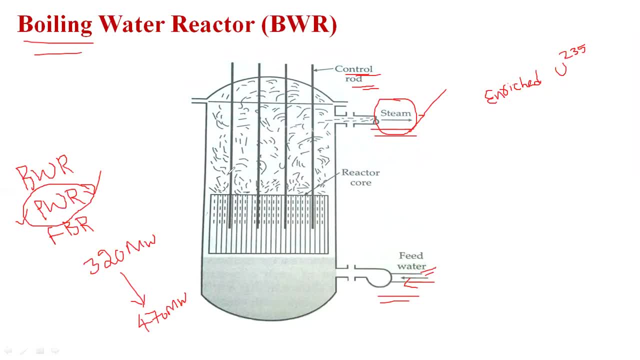 Suddenly. now demand is increased to 470 megawatt, That is, 150 megawatt. the demand is increased within a short interval of time. Within short interval of time, the demand is not fulfilled By using the boiling water reactor. By using the boiling water reactor, 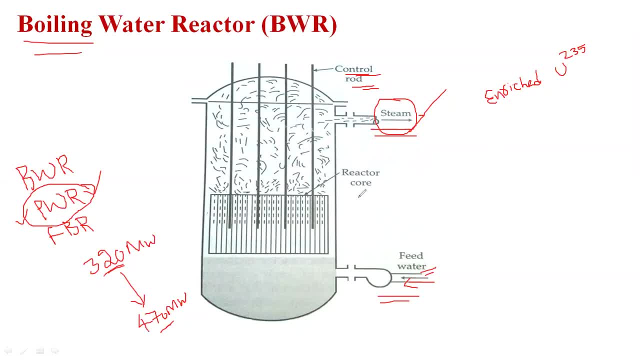 Why it is not fulfilled means Here. they are not used for the heat exchanger That is the moderator we are not using Directly drives the steam turbine. That is the water as well as steam is only taken place in the single place. 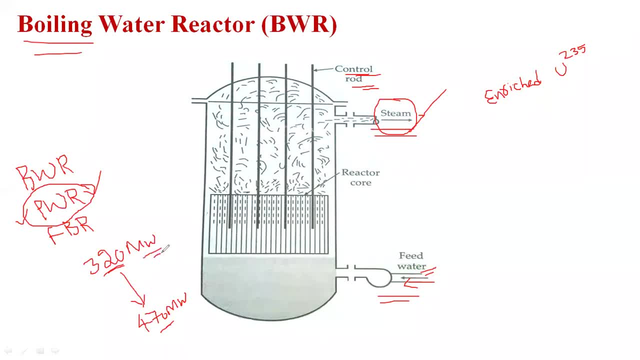 That is, in the reactor itself. Due to that, the efficiency is also very, very less. The efficiency is also very, very less. The advantages: The advantages in that the boiling water reactor is: This reactor does not require heat exchanger circuit separately. Due to that, the cost is minimized. 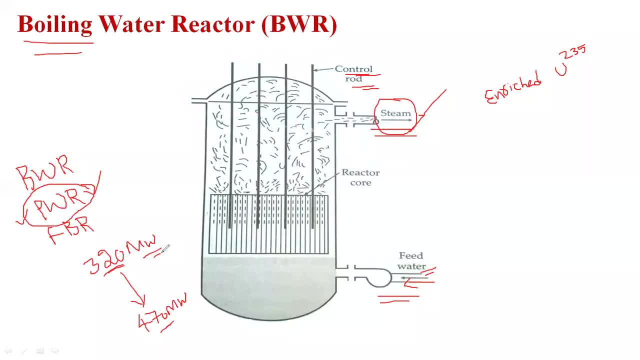 This is the advantage And the thermal efficiency of the reactor plant is considerably higher than the pressurized water reactor. And the major drawback in that the boiling water reactor is In this: the BWR cannot meet sudden increasing in load, Suddenly if the demand is increased. 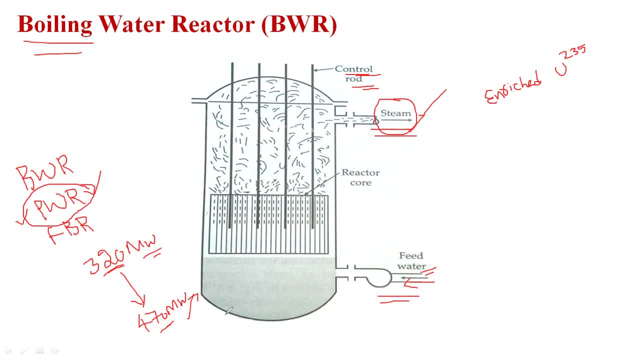 We cannot satisfy it for the demand. within short interval of time, That is, within a minutes Under Here, the radioactive contaminant, The steam, is released in the director. See if any alpha or beta or gamma radiation is released means That directly drives the steam turbine. 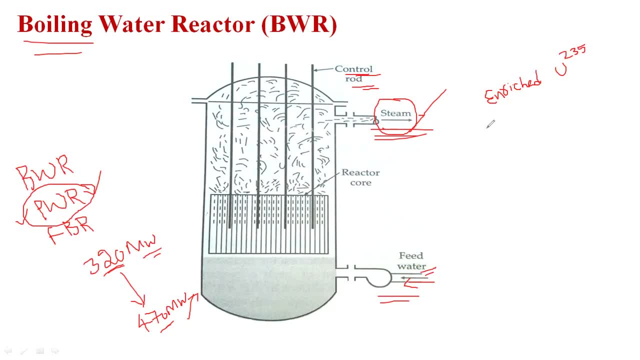 Maximum amount of the steam is wastage in the turbine, Here it collected in the condenser, There it is entering to the atmospheric particle. Due to that, the living, both Living as well as for the non-living organisms, are affected, And these are the drawback of the boiling water reactor. 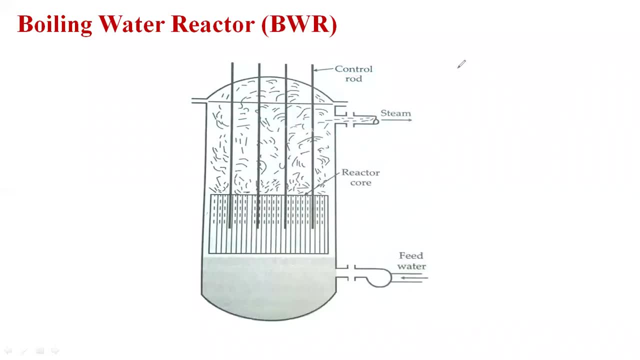 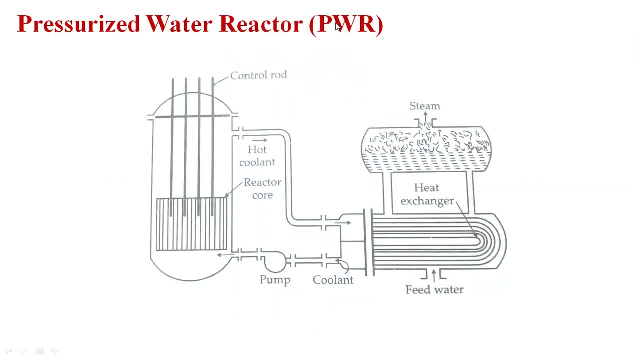 Here. they are not used for the heat exchanger. For that purpose it is not preferred that much. Due to that it polluted to the environment due to the radioactive substances. And the second one is the pressurized water reactor. It is represent for the PWR. 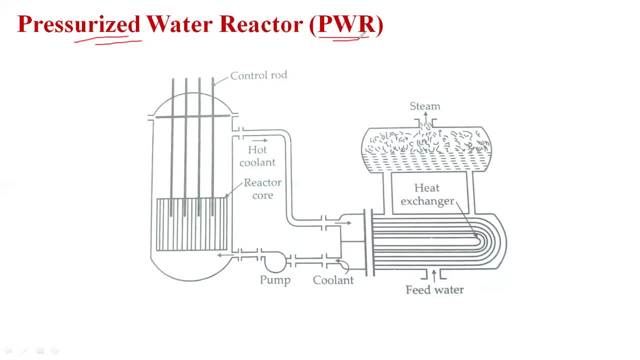 Pressurized water reactor is represent for PWR Here In the pressurized water reactor it is nothing but a thermal reactor. The pressurized water reactor is nothing but thermal reactor Maximum, all the nuclear power plant. they are preferred for the PWR. 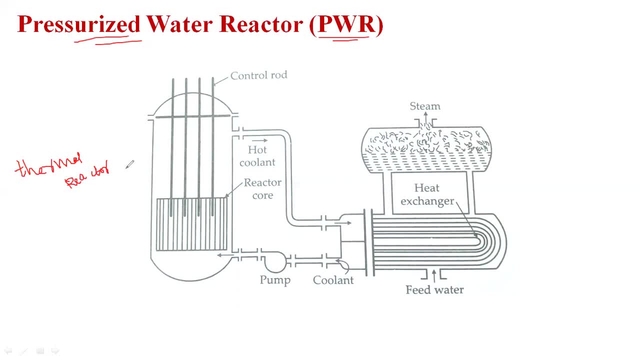 That is the pressurized water reactor. Here the fuel used is enriched uranium. In the pressurized water reactor The fuel used is enriched uranium. That is, uranium 235.. Uranium 235 plus adding one small neutron, We are getting unstable uranium. 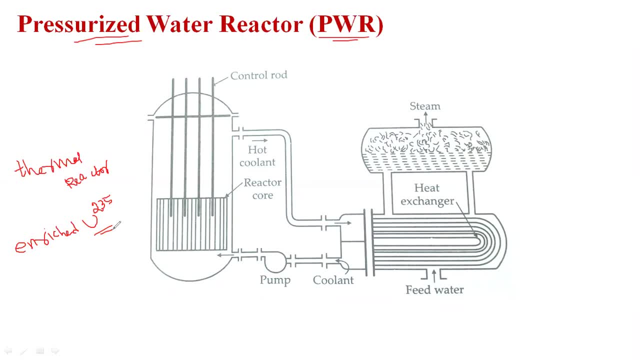 That is uranium 236.. Whenever the fission process is taken place, it is bombarded And, due to the nuclear fission, The splitting of heavy nuclei into two or more small nuclei, That is, splitting into two small nuclei, That is for the latinum. 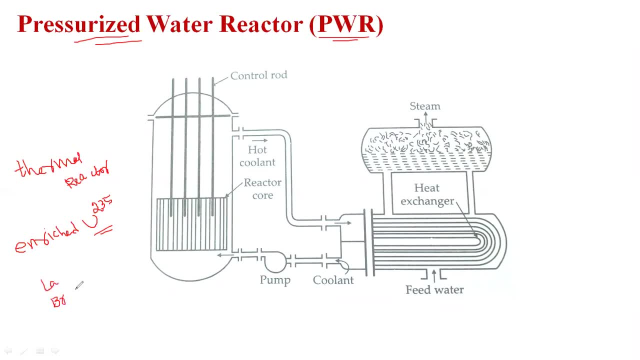 Another one is nothing but the bromine, And it releases for the three small neutrons And releases for the three small neutrons. Due to that, The chain process is taken place, But here the fuel used in the pressurized water reactor is enriched uranium. 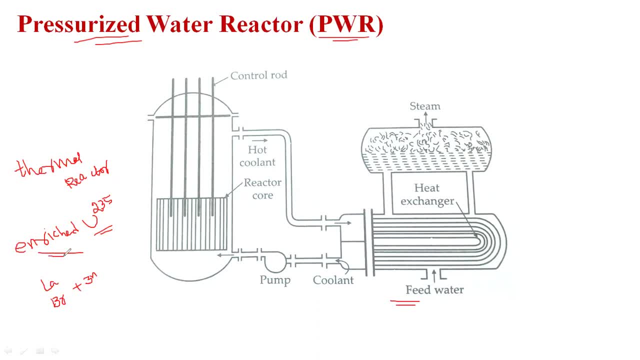 Uranium 235. Here the water is used for both moderator as well as for the coolant, But here it is nothing but the nuclear reactor. And separately they are used for the heat exchanger, Here used for the two parameters. The fed water is given into the heat exchanger. 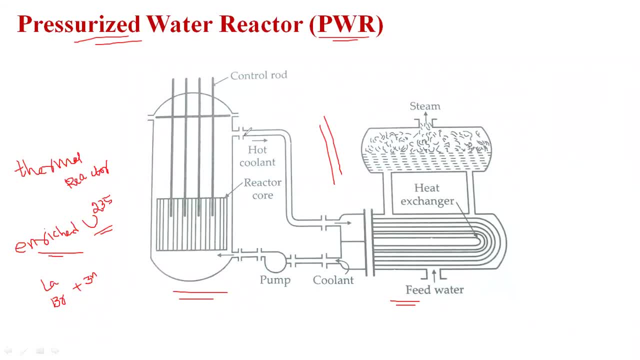 In the tube. whenever the fission process is taken place, The heat of hot coolant is flowing into the tube Surrounding the water. This, the water, converted in the form of steam. Here the separate chamber is there, One is nothing but the water chamber. 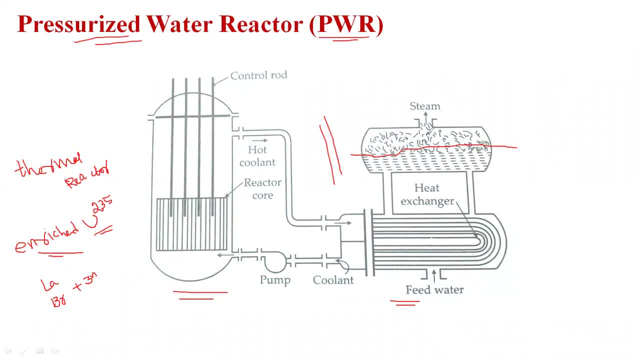 Another one is nothing but the steam chamber, The generated steam. This is nothing, but without the moisture particle. Directly the steam drives, the steam turbine. It can convert the steam energy into mechanical energy. In this, This is the pressurized water reactor. 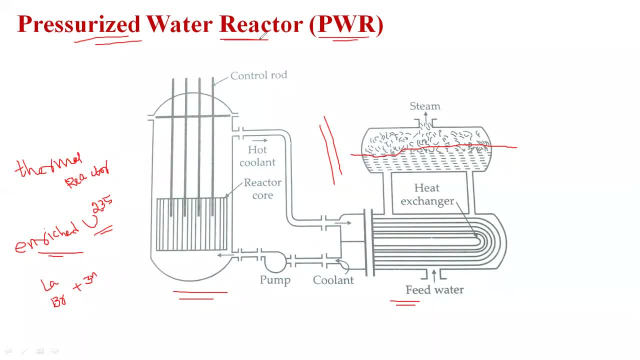 Within short interval of time. Suddenly the demand is increased. We can fulfill the demand By using this, the pressurized water reactor, And the efficiency is also maximum. The efficiency is also maximum, Suppose if any radioactive substance is released here, It is not directly mingle into the heat exchanger. 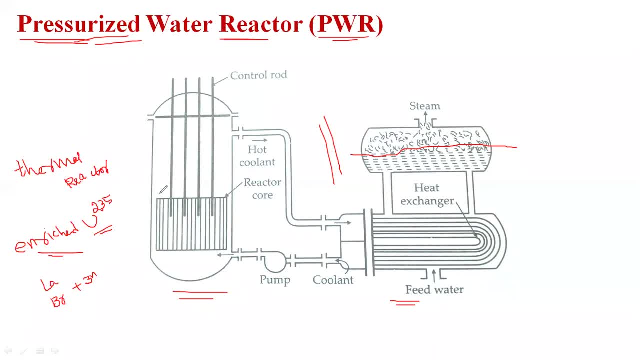 It is not directly mingle into the heat exchanger, In this the reactor core itself, observed in the shielding, Observed in the shielding, And here the pump circulated the water. This is the pump circulated. the water At used is high, That is nothing. but the pressure is nothing but 140 kg per centimeter square. 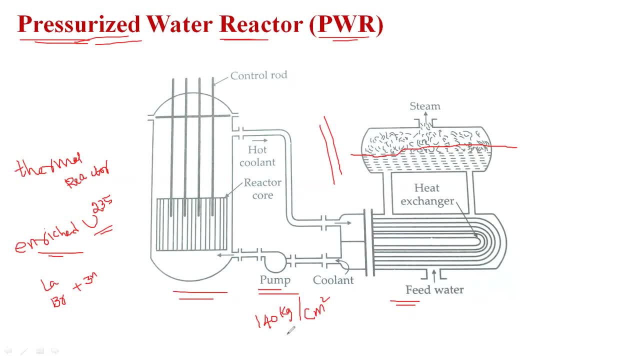 That is, the water is circulated. in the nuclear power plant The pressure is 140 kg per centimeter square And liquid state the temperature is 240 degree centigrade. Here in this, the heat exchanger, The temperature is maintained from 240 degree centigrade. 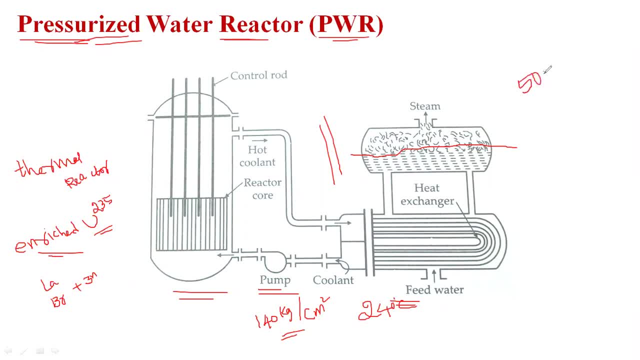 But in the nuclear power plant Temperature is maintained from 250 degree centigrade to 500 degree centigrade. The temperature is maintained from 250 degree centigrade to 500 degree centigrade, But in the fed water the maintain the temperature is maintained from 240 degree centigrade. 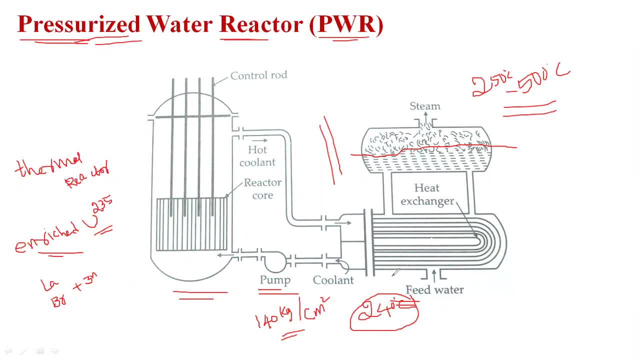 Here in the pressurized water reactor. The advantages is the reactor is compact in size Comparing to the boiler water reactor And the water is used for coolant purpose. Moderator. And the cost is very, very less comparing to the boiler water reactor. 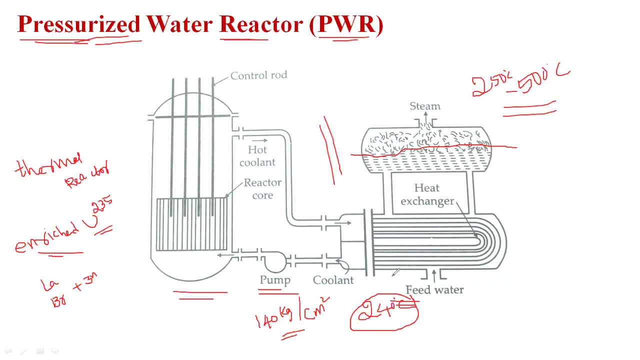 As well as for the fast beater reactor, And here the load is increased. in the pressurized water reactor Supplied is more power Suppose. the suddenly demand is increased Suddenly. the demand is increased Within a minute. we can satisfy for the demand. 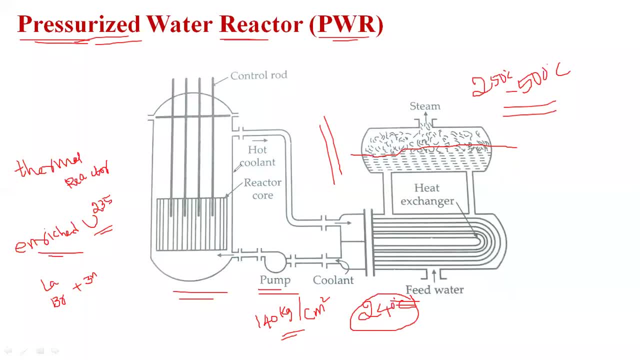 But this feature it is not available in the boiler water reactor But maximum all the nuclear power plant. They are prepared for the pressurized water reactor And the drawback is occurrence of heat losses in the heat exchanger. Again in this the heat exchanger, due to 10 to 15 percentage of the steam is wasted. 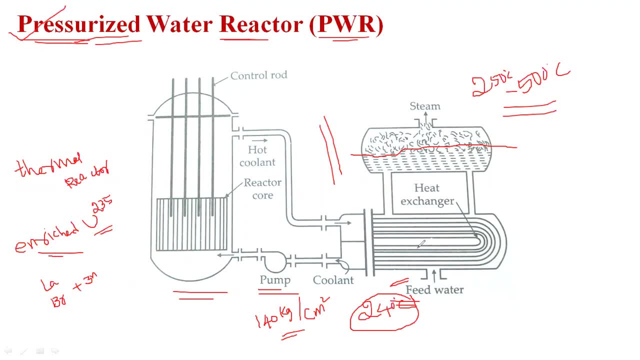 That is the major drawback, And thermal efficiency of the pressurized water reactor is low. That is, 20 percentage of maximum. 15 to 20 percentage of the steam is wasted Due to that. the thermal efficiency is minimized. Thermal efficiency is minimized. 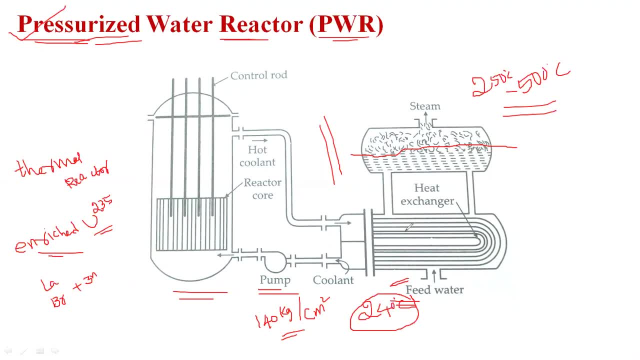 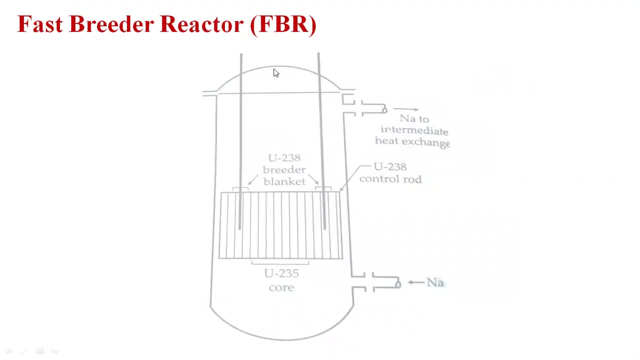 And one more thing: The safety precautions it should be taken. comparing to the other type of reactors, Other type of reactors. The next one is fast breeder reactor, In the name itself, available. There is nothing but the fast breeder reactor. Here the power generation is maximum. 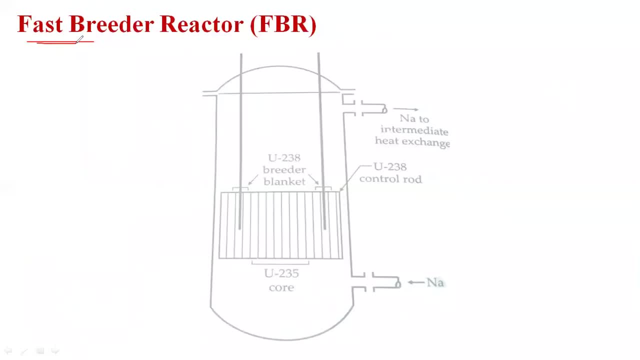 In the name itself mentioned, That type is nothing but the fast breeder reactor. Here in the fast breeder reactor They are not used for the moderator, They are not used for the heat exchanger Only they are used for the reactor core. 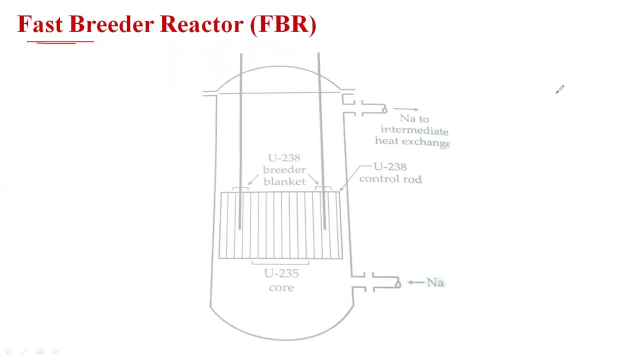 Once they are generated, the steam That directly drives the steam turbine. But in the previous cases they are used for the water. But here they are used for the That is nothing but the Sodium. Here they are preferred for the material, That is, they are used for enriched uranium. 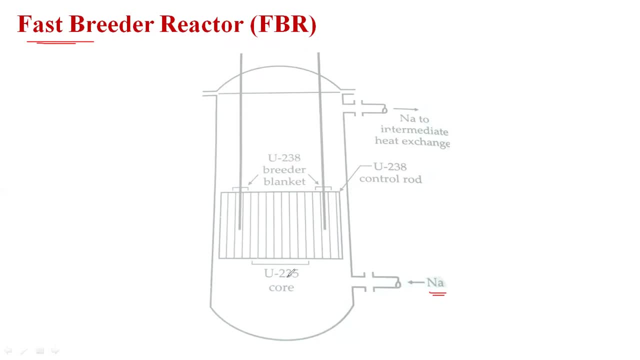 That is uranium 235. They are used for uranium 235.. Once the fission process is taken place in the control rod, Whenever the control rod is pushing to the Fission Push into the core, Observe the sum amount of the fission process. 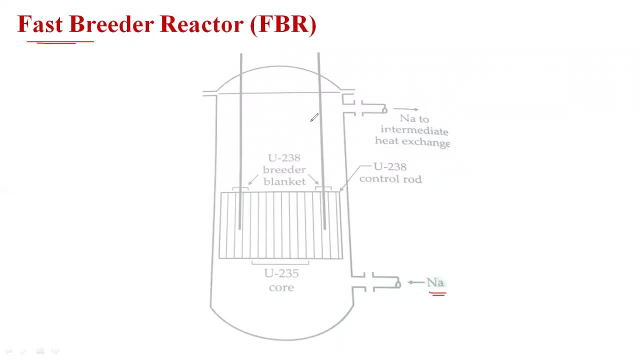 It releases for the small amount of neutrons. Due to that, the power generation is minimum. Whenever the control rod is pull out, More number of the fission process is releases. Due to that, the power generation is maximum. The power generation is maximum. 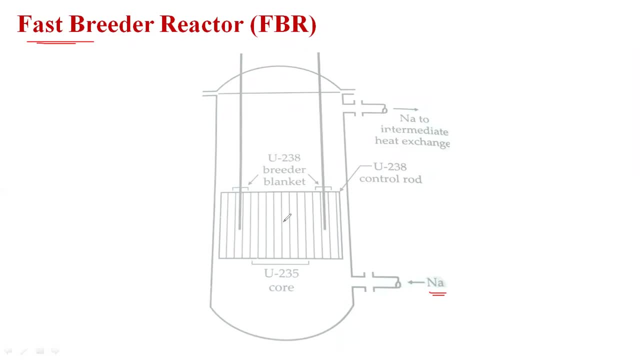 And one more thing Here. they are not used for the moderator. And then heat exchanger. We cannot control for the fission process. Here the power generation is maximum. More number of the fission process is released, More number of the fission process is released. 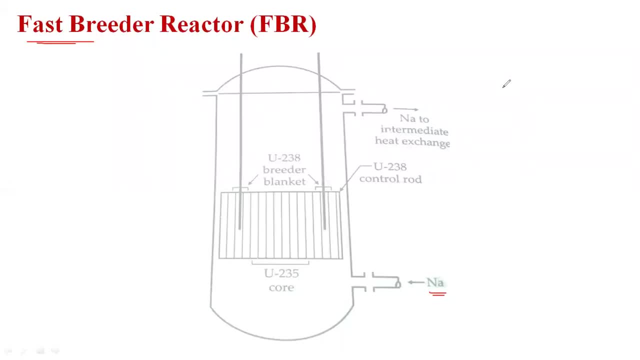 We cannot control the power generation. We cannot control the power generation Due to that. here the drawback is Huge amount of the fuel is required. The fuel consumption is maximum Here. already we know that in the nuclear power plant The fuel cost is very, very high. 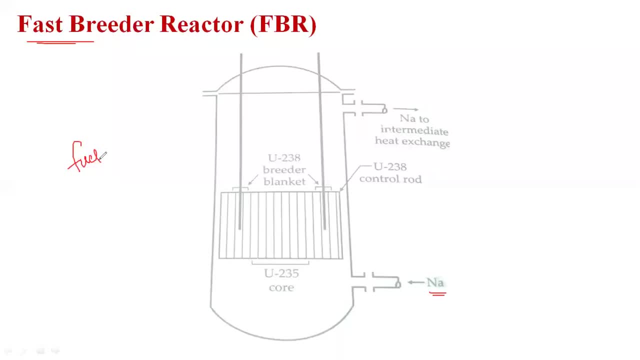 The fuel cost is Very, very high comparing to the remaining other conventional power plant. The fuel utilization is maximum in the fast beater reactor And another one. It is not observed for the moderator as well as for the heat exchanger, Due to that directly the radioactive substances. 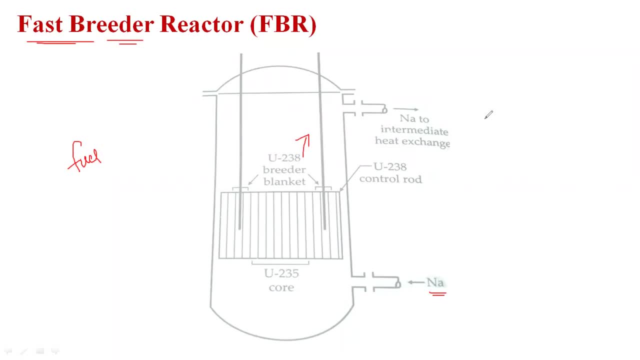 Entering into the turbine, Entering into the atmosphere. Due to that, it polluted to the environment. It polluted to the environment For that purpose. The fast beater reactor: they are not preferred that much of thing Comparing to these three. 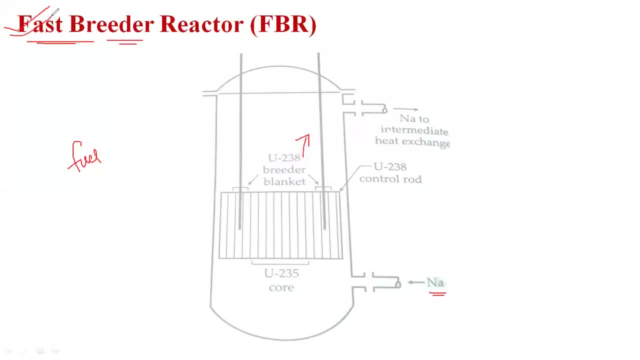 Boiler water reactor. Pressurized water reactor, Another one is for the fast beater reactor. They are preferred only for the pressurized water reactor. They are preferred only for the pressurized water reactor. The differences between the nuclear fission and the nuclear fission. 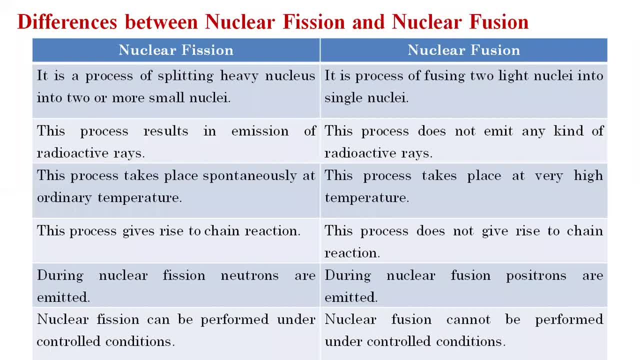 There are two processes taken place. One is for the fission process, Another one is for the fusion process. Already- this last class, we have discussed The nuclear. the fission means The splitting of heavy nuclei Into two or more small. nuclei is nothing but the nuclear fission. 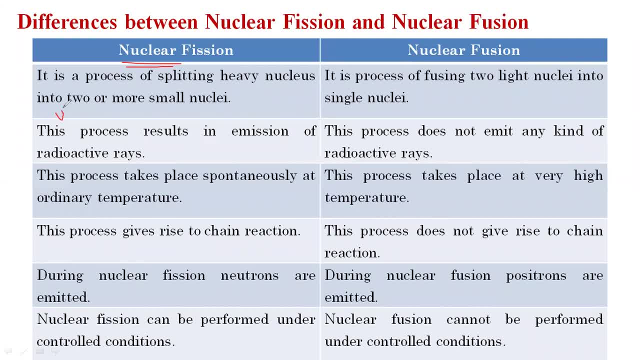 That is the example here we have taken for Uranium 235. Uranium 235 They are adding, and small neutron They are getting the unstable uranium 236. That is, this is nothing but the heavy nuclear. The splitting of heavy nuclei into two or more small nuclei is nothing but the nuclear fission. 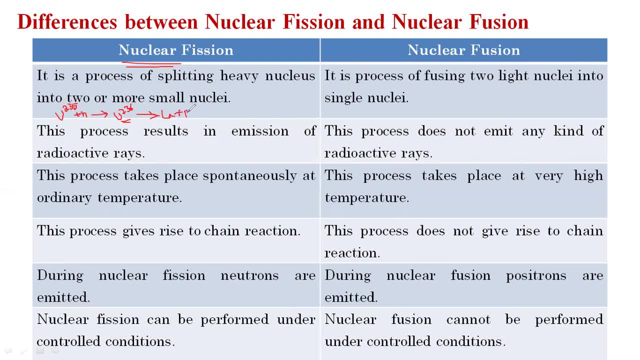 That is, It releases splitting of two small nuclei. One is nothing but the latinum, Another one is for the bromine and it releases for the three small neutrons. It releases for three small neutrons Nothing but the nuclear fusion means the splitting of heavy nuclei into two. 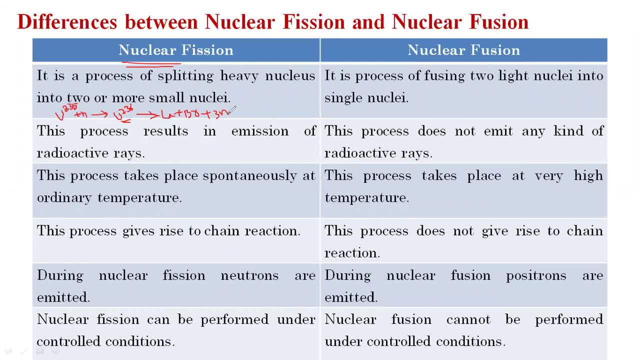 or more. The small nuclei is nothing but the nuclear fusion. But in the nuclear fusion means lower and then higher mass energy. It is gathered into the central particle. Finally it releases for the single nuclei Here the example we have taken for the two. 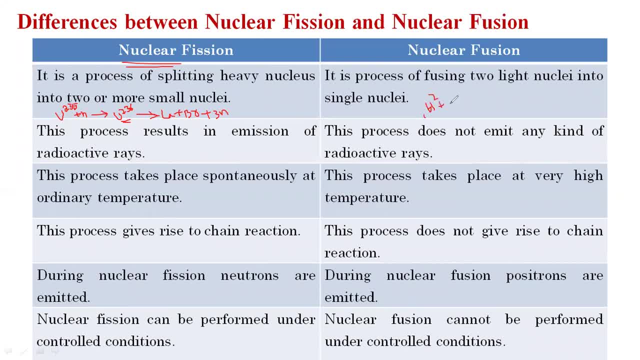 hydrogen element, That is, the lower as well as for the higher, the mass value Bring into the central particle. Finally, it releases for the helium. This is called as the nuclear fusion And in the nuclear, the fusion process the result is the emission of the radioactive. 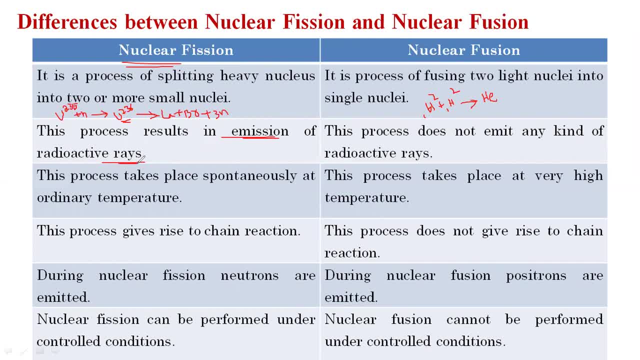 rays Process of resulting the emission of the radioactive rays, But in the fusion process it does not emit any radioactive rays. It does not emit any radioactive substances, Radioactive rays in the sense it releases, for the alpha rays, beta rays, Another one. 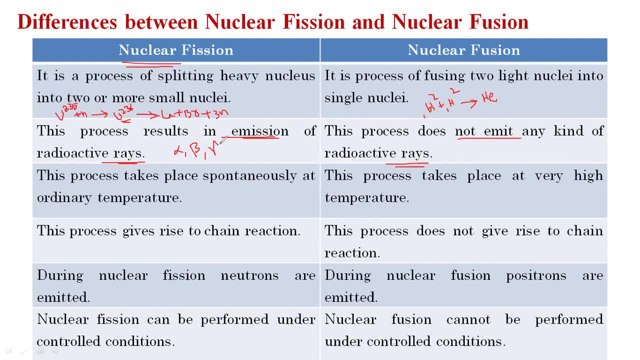 is for the gamma rays Generally in the alpha radiation means it is in this alpha radiation. it is not affected for the human being. It is taken place in the reactor itself, Taken place in the reactor itself. It is taken place in the reactor itself. It is taken place. 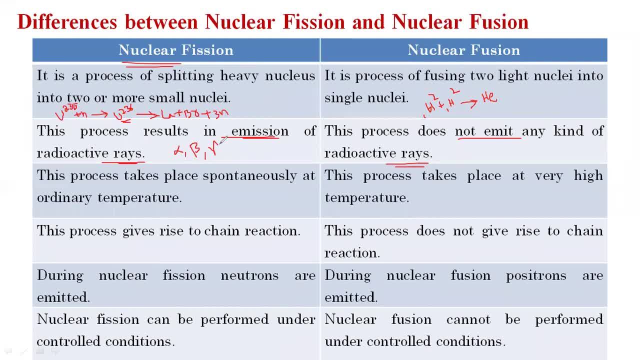 in the reactor itself. It is not entered into the open atmosphere. due to the, the effect is very, very less, But due to the beta and then gamma radiation it is affected for the whole living as well as for the non-living organism. Enter into the open atmosphere. 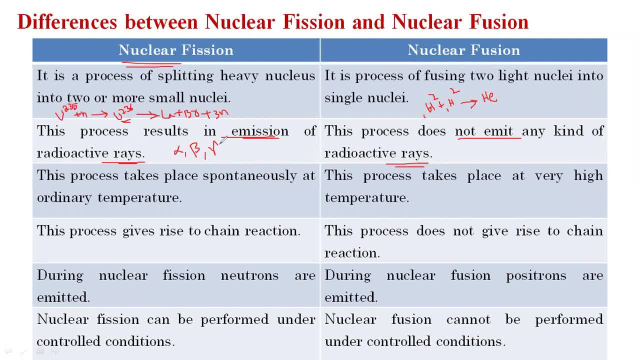 Due to the beta rays, the human being affected, for the cancer, A number of cancers have appeared And due to the gamma radiation DNA problem, the inspiration problem, skin diseases have appeared. In this, the fission process, the emission of the radioactive rays, But in the fusion, 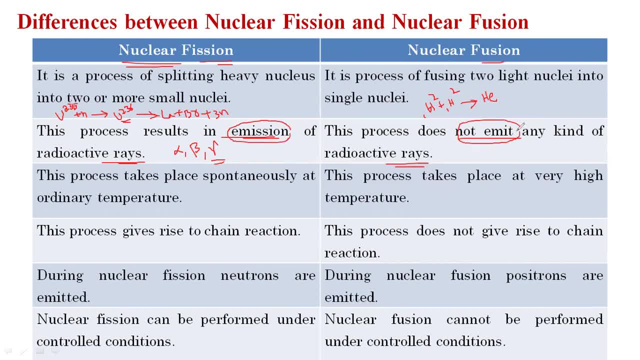 process. it does not emit any kind of radioactive rays And in this nuclear fission it is operated under ordinary temperature. Under normal temperature the process is taken place, But in the fusion process the heavy temperature is required. In fusion process heavy temperature is required. 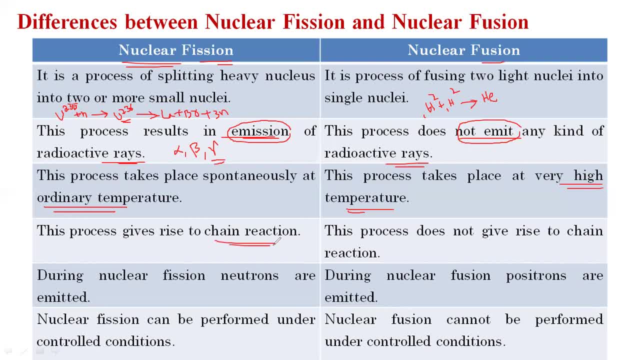 And in the nuclear fission chain reaction is taken place, And in the nuclear fission It does not produce any chain reaction. The chain reaction means it is bombarded, That is, the splitting of heavy nuclei into two or more small nuclei. 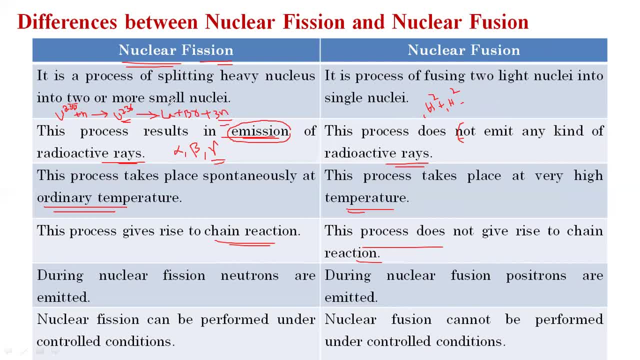 Here, three neutron is formed. Again we are adding one more small neutron. Again the chain reaction: Again 3 plus 3 into 3.. Again, 9 neutrons are released. Again it is bombarded. 27 neutrons are released. 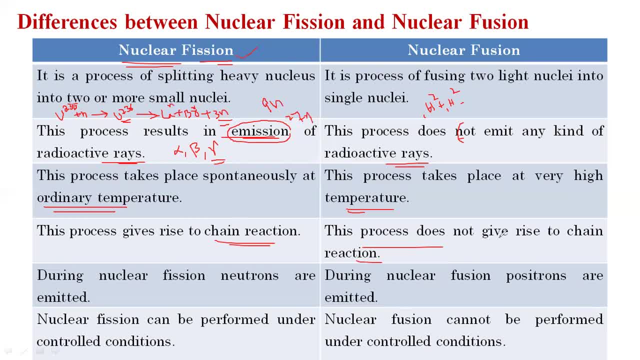 That is, chain process is taken place in the fission process And it does not produce any chain reaction in the nuclear fission. During nuclear fission neutrons are emitted, But in the nuclear fission positrons are emitted. Positrons are emitted. 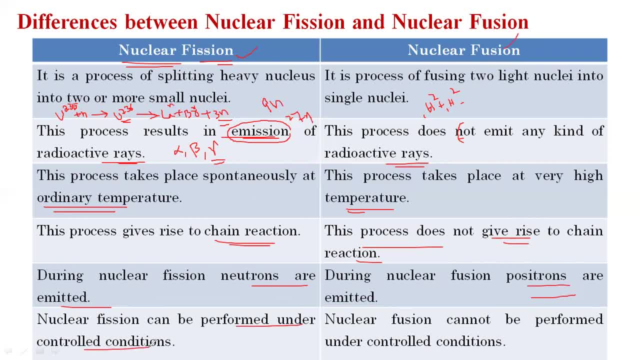 And in the nuclear fission it can be performed under controlled condition. It can be performed under controlled condition, But in the nuclear fission it cannot be performed under uncontrolled condition. It cannot be performed under Uncontrolled. This is the differences between nuclear fission and the nuclear fission. 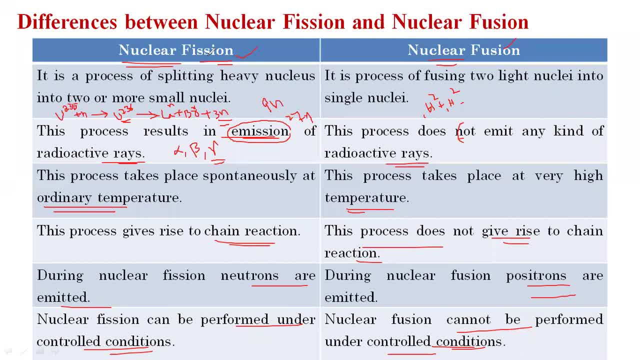 Simply, the nuclear fission means splitting of heavy nuclei into two or more small nuclei is nothing but the nuclear fission. The best example is this: operation under 35 conditions. If the nuclear fission can be performed under 35 conditions, Here I am giving the example of only one condition. 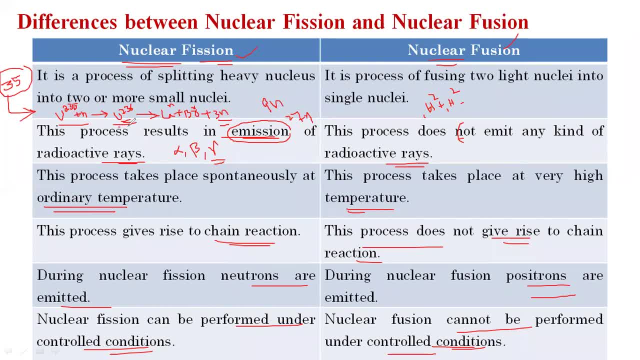 That is uranium-235, is adding one small neutron. We are getting one unstable, uranium-236.. Once it is bombarded, that is, fission process is taken place. it releases for the two small nuclei, One is nothing but the latinum. 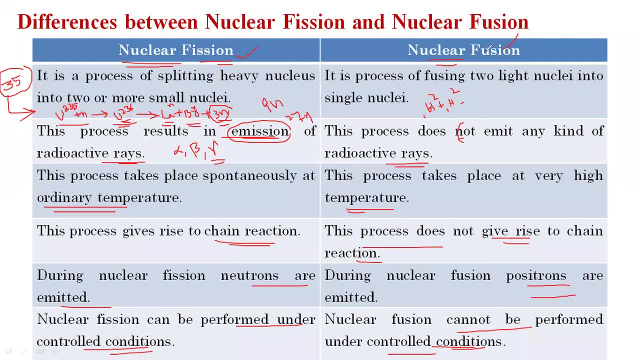 Another one is for the bromide And it releases for the three small neutrons A nuclear fusion means that it is lower, as well as for the higher the mass value. Bring it to the center particle. Finally, we are getting for single nuclei. 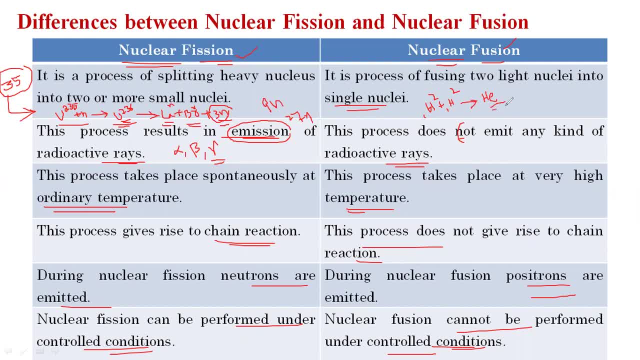 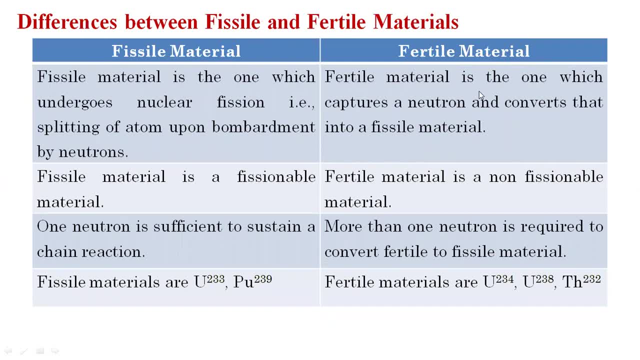 That is, two hydrogen elements. The output we are getting in the form of helium. The output we are getting in the form of helium. Next, the differences between Fissile and then fertile material. The differences between the fissile and then fertile material. 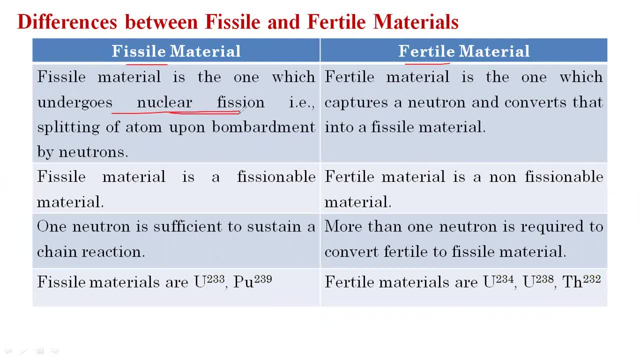 That is, the fissile material, is undergoes in the nuclear fission process The splitting of heavy nuclei into two or more the small nuclei, That is, whenever the bombarded in the fission process, That is, the uranium-235.. 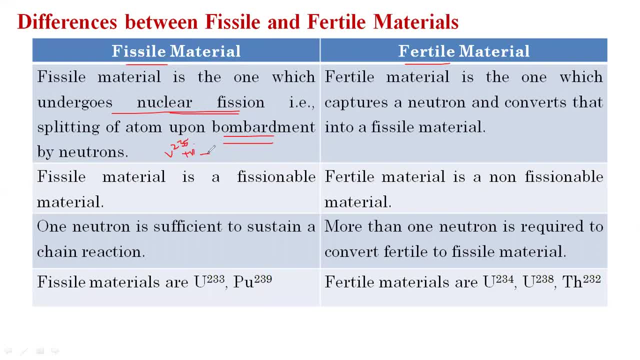 Uranium-235.. We are adding one small neutron That is, unstable, uranium-236.. Once the bombarded, the fission process is taken place, We are getting two small nuclei. One is nothing but the Latana, Another one is for the Bromine. 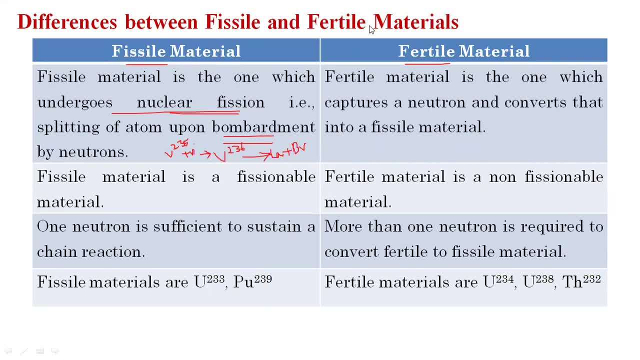 Another one is for the Bromine. But in the fertile material it is captured in neutron and converted that into a fissile material. That converted into a fissile particle And the fissile material is a fissionable material. That is nothing but the burning process. 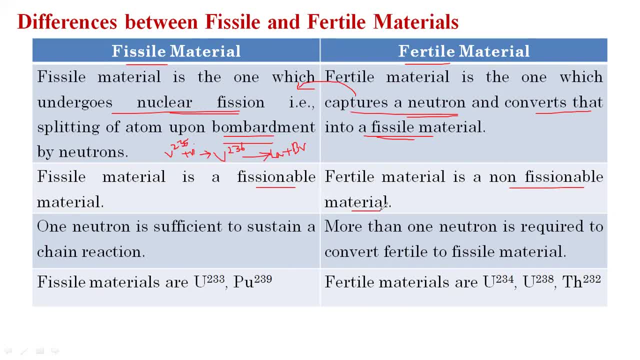 But the fertile material is non-fissionable material, That is, non-burning material. This converted into the fissile material, And in the fissile material one neutron is sufficient to form a chain reaction. One neutron is sufficient to form a chain reaction. 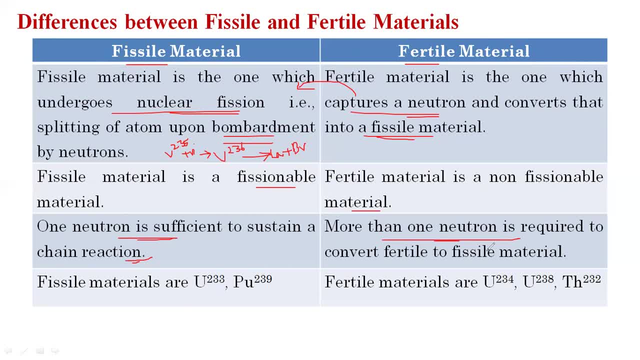 But in the fertile material more number of neutrons is required to convert the fertile to fissile material, Fertile to fissile material. That is here we are using uranium-235.. We are only adding for the one small neutron. 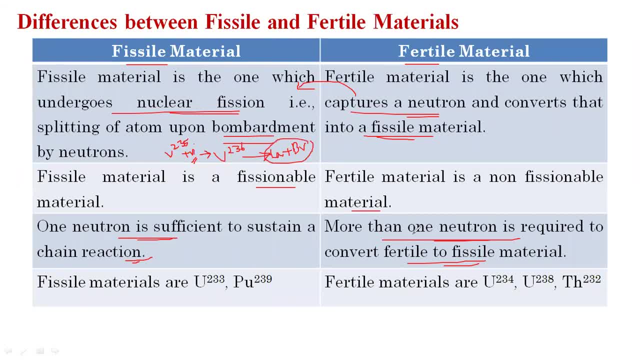 We are getting, for the fissile process is taken place, But here the fertile into the fissile material we are getting more number of neutrons. That is, the fissile material is represent for uranium-233 and plutonium-239.. Fertile material means uranium-234, uranium-238 and thorium-232. 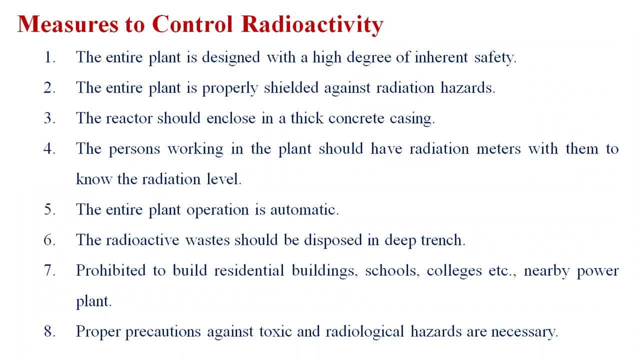 Actually in the nuclear power plant. the major drawback is it releases for the radioactive substances. Due to that, it is polluted to the environment, for both living as well as for the non-living organism. How we can control the radioactive material? What are? 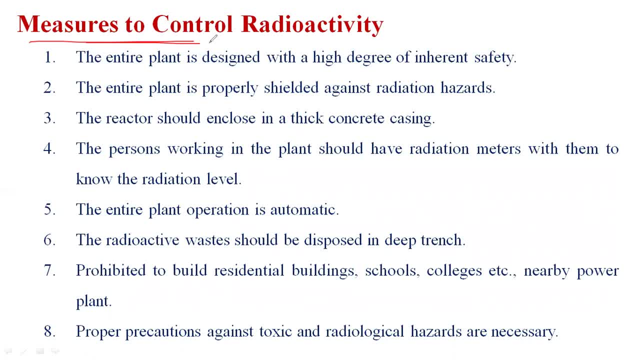 What are the measures we can take to control the radioactivity? The main thing is that the entire power plant is designed with high degree of inherent safety. High degree of inherent safety- It is this parameter taken at the time of construction itself, And the entire plant is properly shielded against radiation hazards. 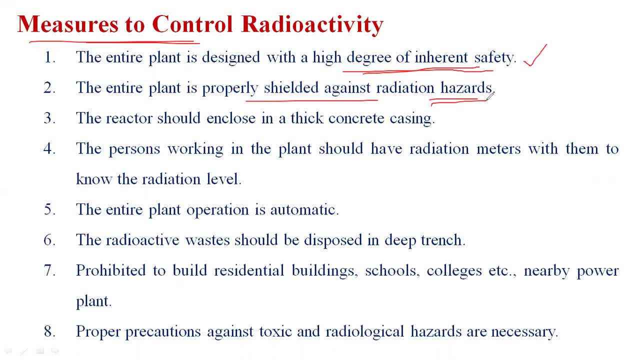 Radiation hazards, That is the alarm signal is taken place. If any, either alpha rays or beta or gamma rays, It releases in the nuclear reactor, automatically shielded in the power plant itself, That is the nuclear power plant. of the construction is the rugged construction and closed tight. 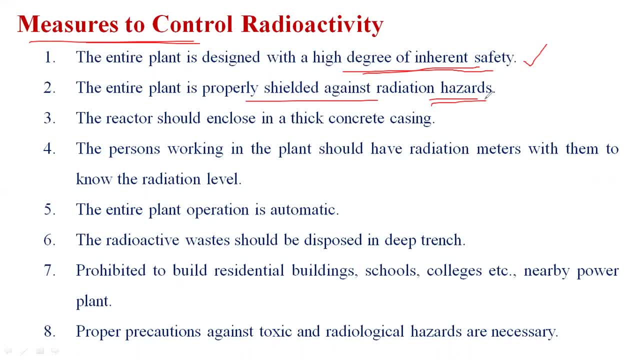 And one more thing: all the nuclear power plant is constructed away from the populated area And the reactor should enclose thick concrete casing, The material in the concrete casing, the material they are used for, the graphite material. These are the various measures. they are considered. 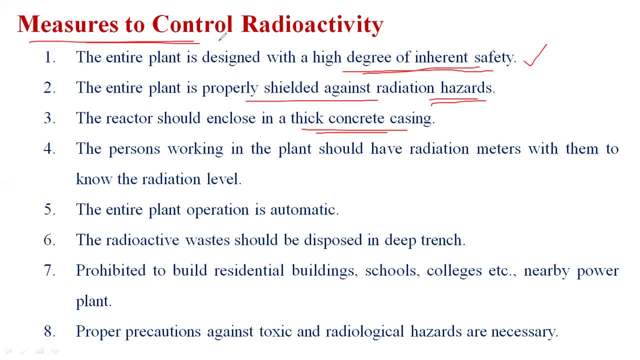 So avoid that. Avoid the radioactive substances And the person working in the power plant. everyone having for the radiation meter always they need to observe the radiation level. Suppose if the radiation is increased means automatically they are shut down for the power plant. 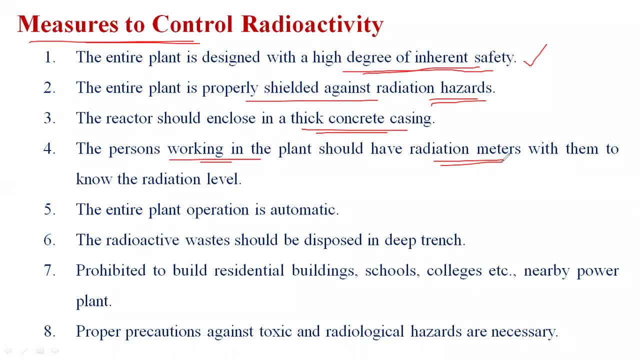 They are shut down for the power plant Automatically is there, another one is for the manual is there And based on the always, they are measured for the radiation meter. One more thing: in the nuclear power plant they are working for all are for well educated person. 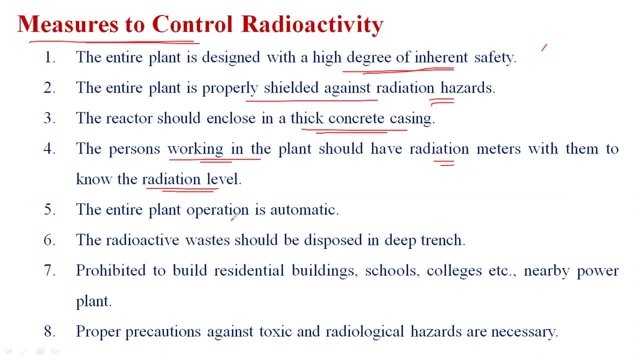 And well trained person. Well trained person And the entire power plant is automatic operation from reactor to up to the end of the alternator, From all the equipment is operated for the automatic operation. Suddenly, if the temperature is increased or any radioactive substances is entered, automatically they measure in the radiation level. 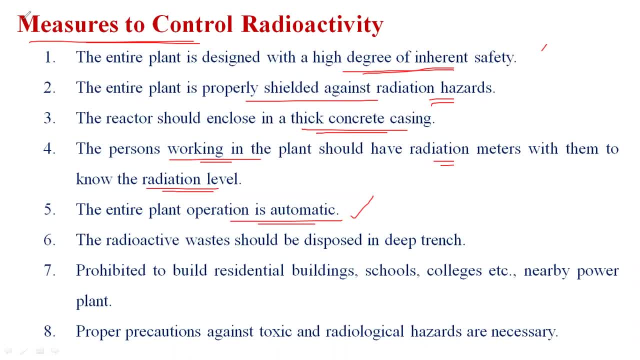 Automatically the plant is also shut down. Like that we are designed for the nuclear power plant And the major drawback is the radioactive substances can be collected in deep tunnel. So this is the challenge which we have to overcome. collected in a deep trench, That is, the wastage particle is collected. that is sending to the 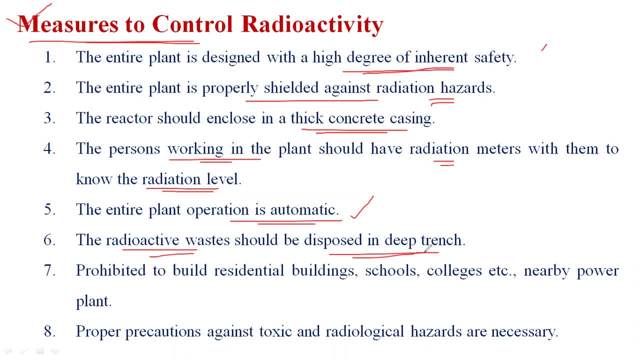 deep trench. Every twice a year we are shut down for the power plant 30 to 60 days, that is, 1 to 2 months. At that time we are removing these radioactive substances and send it away from the populated area, away from the environment. And the major thing suppose, if any accident 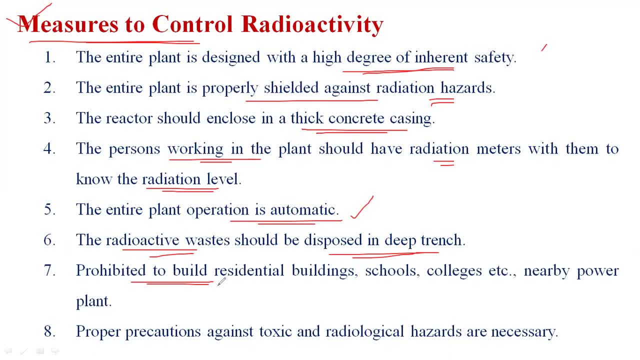 is taken place, the effect is maximum and the losses is also more. For that purpose it is prohibited to build, That is, the power plant can be constructed away from the residential building, away from school, colleges and somewhat nearby the lower center. And proper precaution. 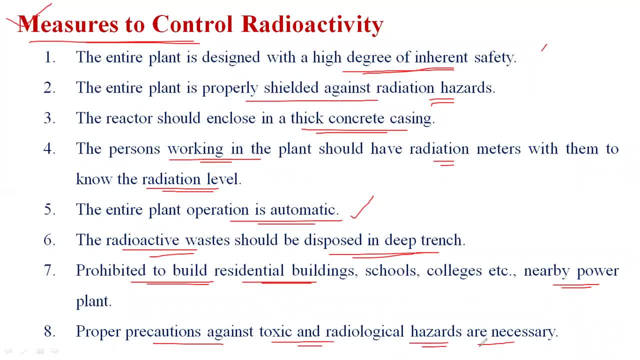 against toxic and then radiation hazards and we need to measure for the nameplate details. Some of them are very important At that time. the industrial visit persons are coming, the auditing is going on. We need to mention all the parameter in the display boards. These are the various measures taken. 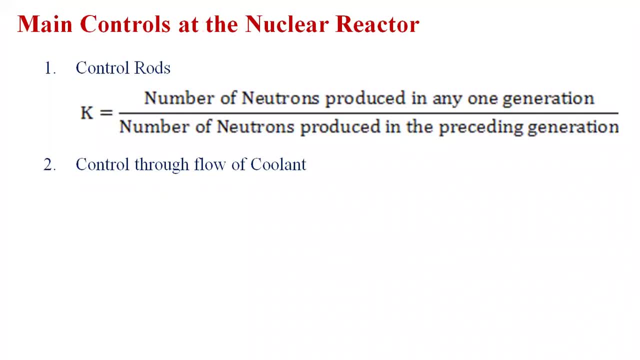 in the to control radioactive substances And main control of the nuclear power plant. there are two controller is there? One is nothing, but with the help of control drum, another one flow of the coolant. Actually, in that the whole power plant, the nuclear power plant, can control based upon the control. 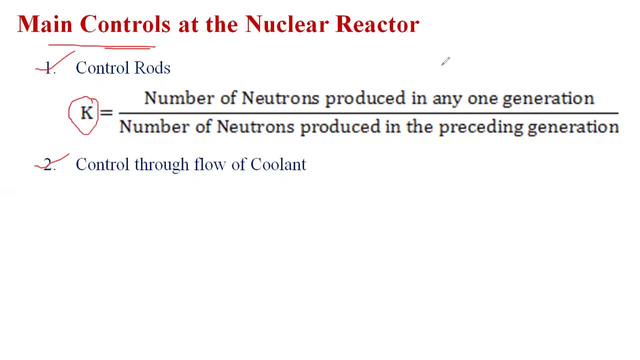 drum. So this is a for a Position a And there being at that particular where there is no host突, praised the unit energy content'm is given in relationship to the unit concept here as following: And Than there should be an over- supposition that virtual sontact is 0, the Nse dualA. 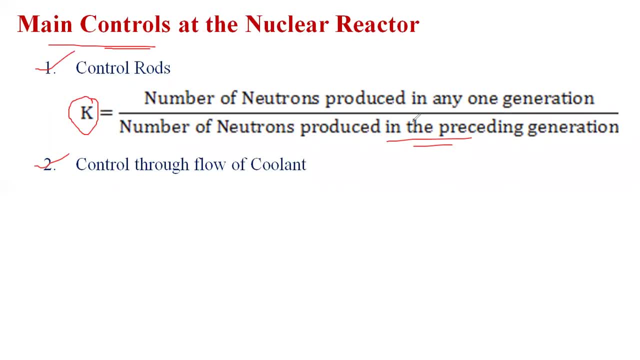 govern the ratio of energy is 대 ficar in coupeств. These were an oppressor of k factor. This represent for the k factor. It is defined as the ratio Number of neutrons produced in any one generation by number of neutrons produced in the frieding generated. Actually, if you go for take for any of the power plant, they run for the single generator, They go for the paternal operation. Either two generating system or four or eight generation system can able cover each one. For this, in single generations how much the neutrons is produced divided? 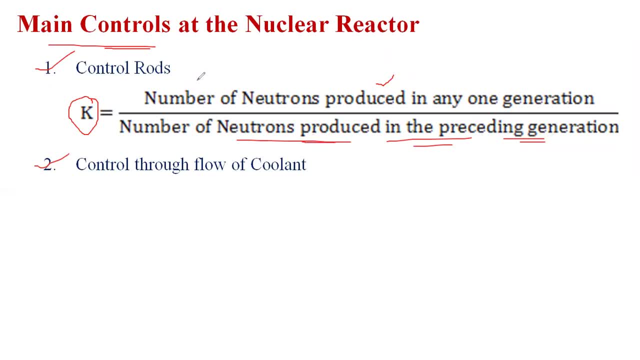 in the preceding generator. That is all generator Under normal operating condition. that is the k factor. the value is unity. The value is unity Whenever the control rod is pushed towards the core. pushed towards the core, it observes the fission process. It observes. 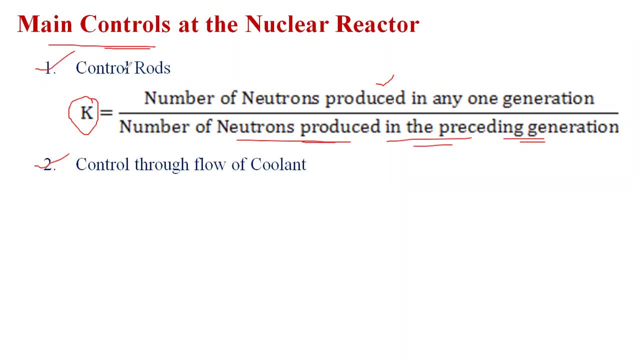 the fission process, Small amount of the neutron is released. That is, the k value is less than unity. The k value is less than unity. Whenever the control rod is pulled out, n number of neutrons are released. n number of neutrons are released At that time. the k value is: 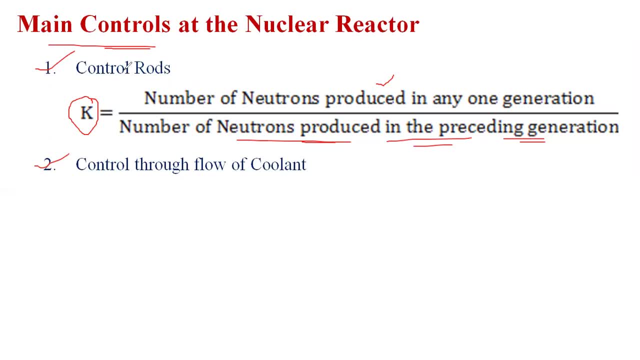 more than unity. The k value is more than unity. Suppose, if the k value is very, very low. if the k value is too low, automatically the plant is shut off. Based upon the control rod only, we are operating for the nuclear power And the second one controls the flow. 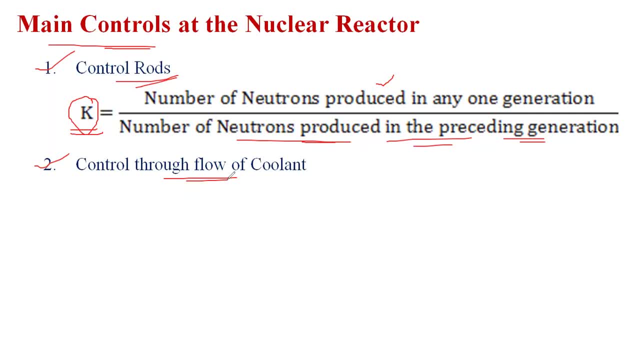 of coolant At constant temperature. the power output is proportional to the rate of flow of coolant The nuclear power plant. these are the two main controls. We are controlling the nuclear power plant With the help of the control rod. another one is for the control through. 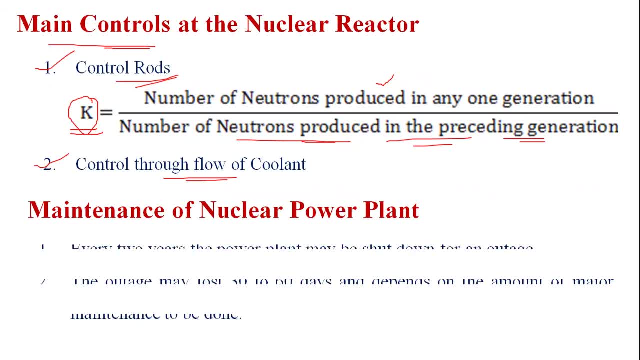 flow of coolant And the maintenance of the nuclear power plant generally in the nuclear power plant every two years one the plant shut down for the outage purpose, That is, under operating condition. we cannot any of the maintenance taken place in the nuclear 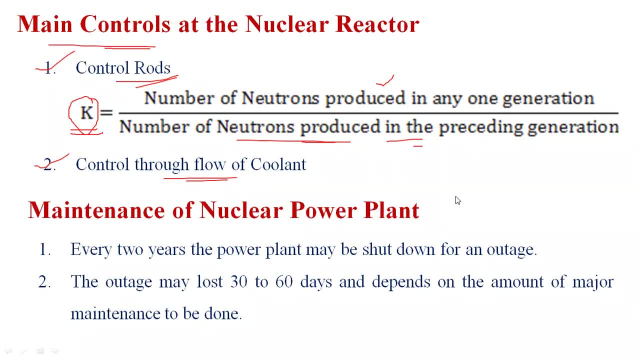 power plant. every twice a year they are shut down for the nuclear power plant. So this is happening to the nuclear power plant At that time, if you remove from the radioactive substances, if you remove from the radioactive substances, at that time that is the plant.